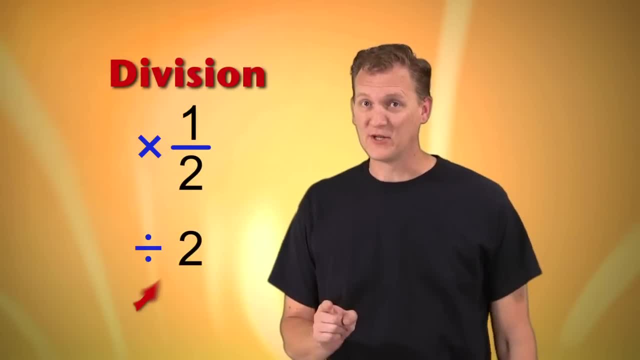 below the fraction 2.. And dividing by 2 is the same as dividing by 2 over 1, because you can turn any number into a fraction by just writing a 1 as the bottom number. right, But look reciprocals. 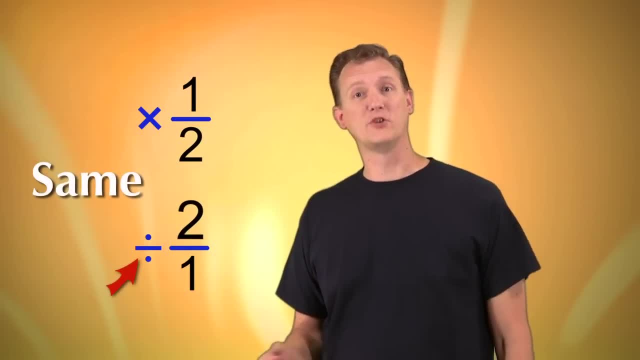 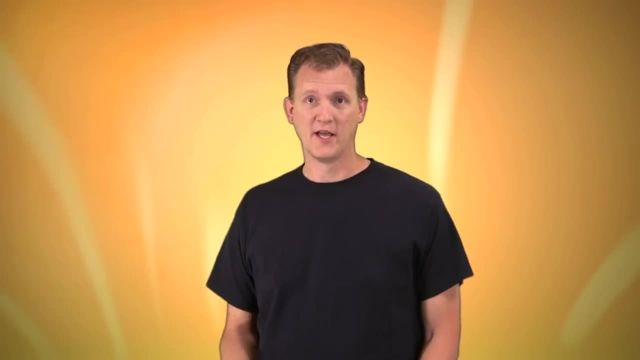 That's why multiplying by 1 over 2 is the same as dividing by 2 over 1.. And it's true the other way around too. So really it's kind of like you NEVER have to divide fractions. You can just rewrite your division problems so that you're multiplying by the reciprocal. 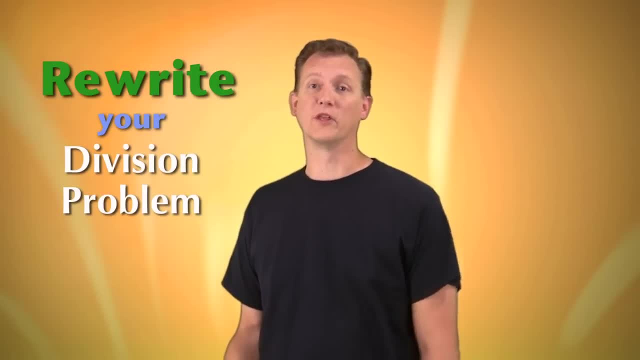 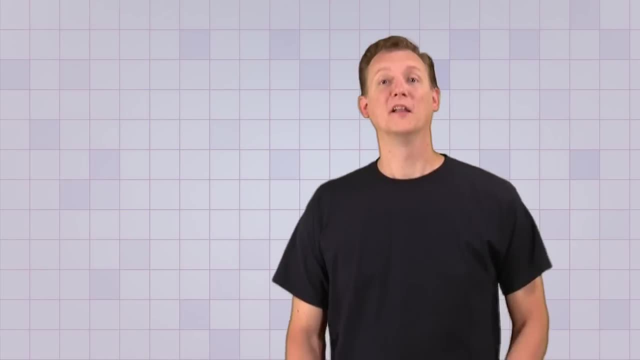 instead. That way you'll get the answer for the original division problem. As always, let's see a couple examples of how this works so you'll really understand. Let's try this problem: 3 over 4, divided by 2 over 7.. 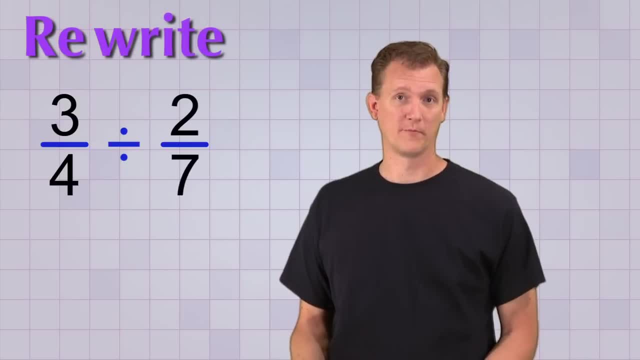 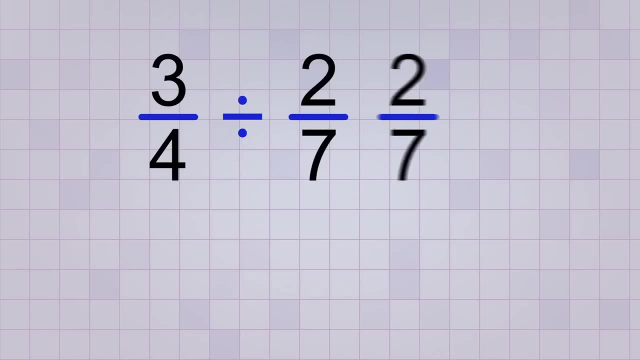 Okay, so the first thing we want to do is rewrite our problem. Instead of dividing by 2 over 7, we can multiply by the reciprocal. instead, The reciprocal of 2 over 7 is 7 over 2.. So our problem becomes 3 over 4 times 7 over 2.. 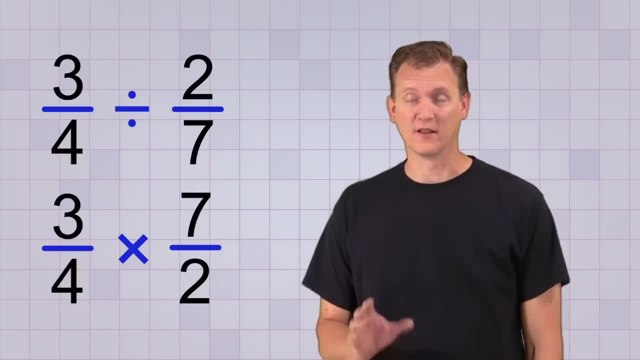 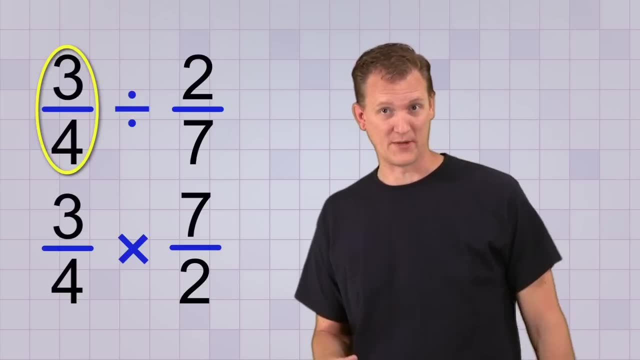 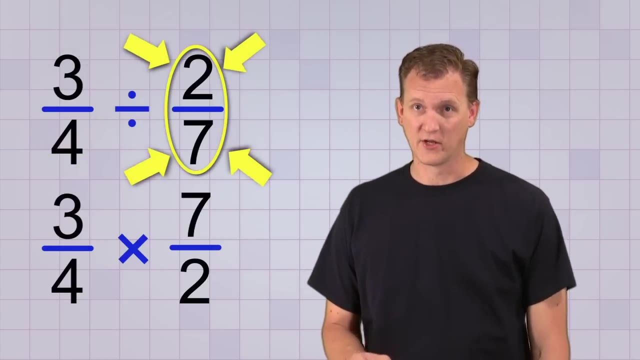 Oh, I should mention a mistake that a lot of students make when they first learn to divide fractions. Sometimes students take the reciprocal of the first fraction, the one that's being divided, or even the reciprocal of both fractions, But you ONLY want to take the reciprocal of the second fraction, the one you're dividing. 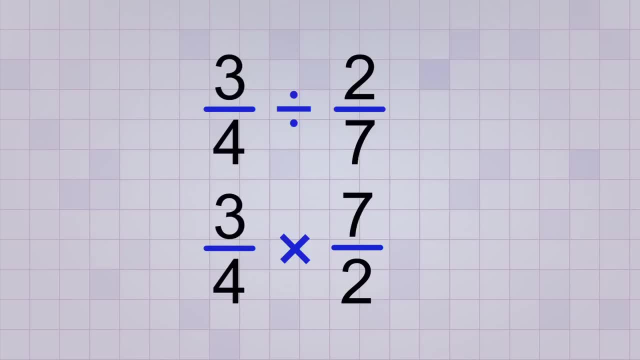 by. Okay, now that our problem has been changed to multiplication, it's easy: Just multiply the tops 3 times 7 equals 21,. and multiply the bottoms 4 times 2 equals 8. And we have the answer to our fraction division problem. 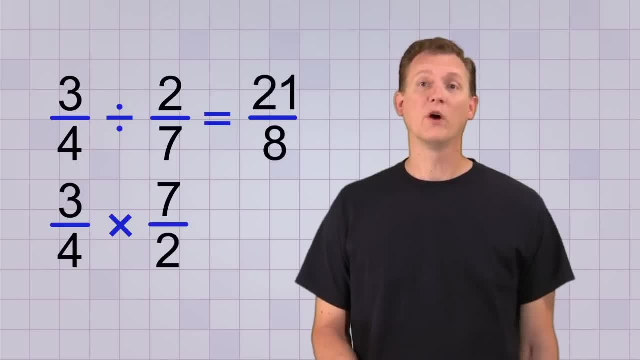 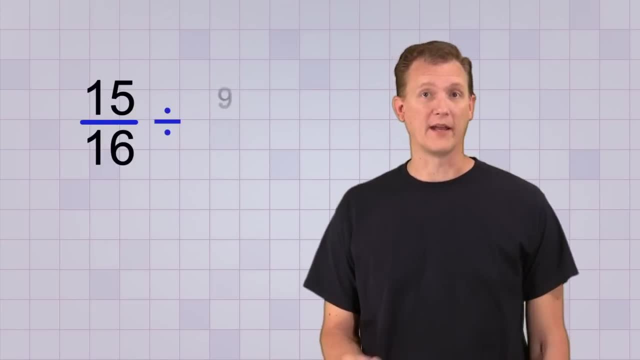 So 3 over 4, divided by 2 over 7, is 21 over 8.. So that's pretty easy. but let's try one more example. Let's try 15 over 16 divided by 9 over 22.. Again, the first thing we want to do is rewrite our problem. 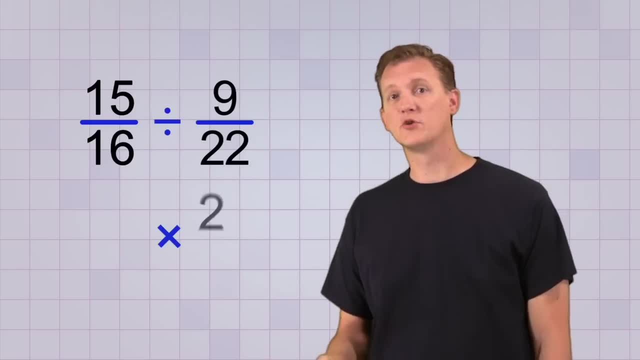 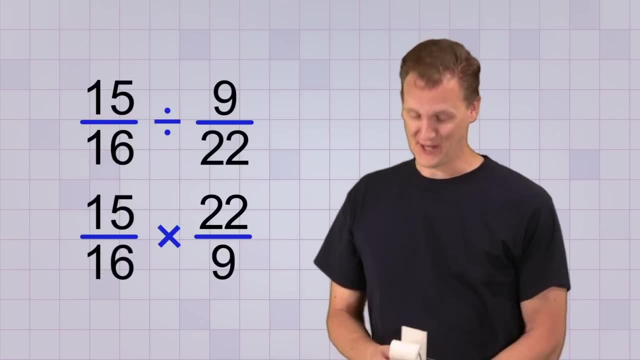 We'll change the divided by 9 over 22 into times 22 over 9.. Now all we have to do is multiply. But since these numbers are kinda big… I'm gonna use my calculator. Let's see here. So we have….